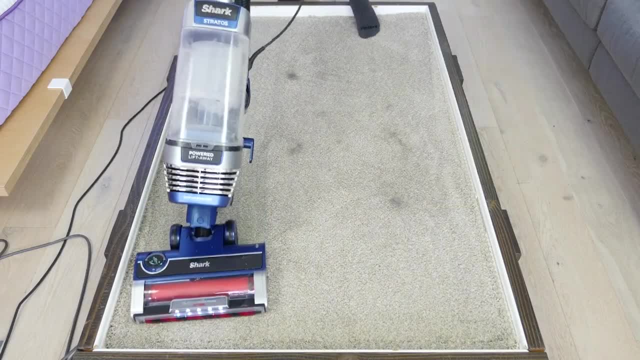 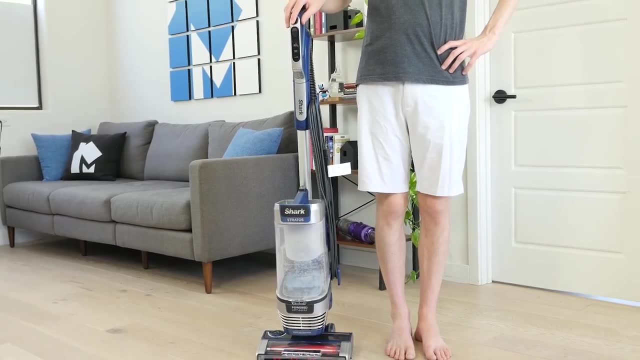 on high pile carpet, but had no issue with pet hair on the same floor type. In addition, the vacuum had no issues with long hair and avoided all hair tangles, Supporting a 0.37 gallon dustbin that's fully sealed with trap allergens and a sufficient 30 foot power cord, the Shark Stratos. 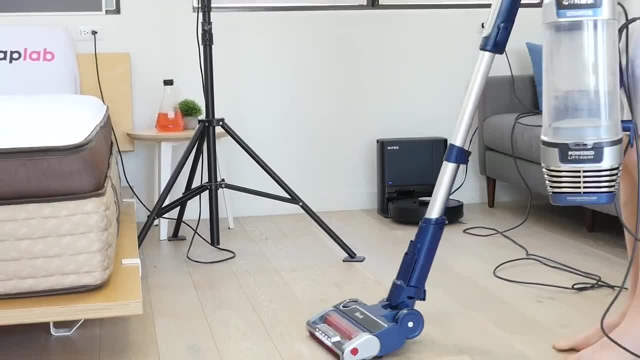 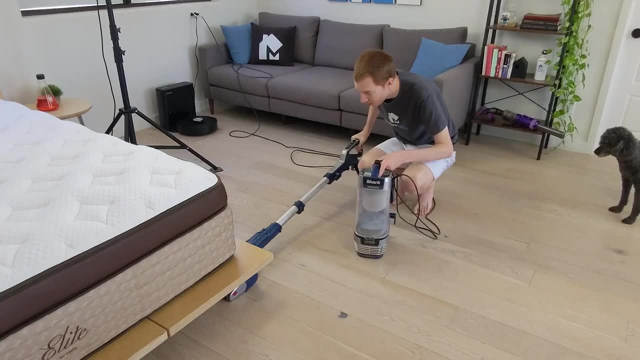 offers capacity and reach. Furthermore, the usability of the Shark Stratos is excellent. It has a lift away feature to act as a canister, vacuum, washable filters for reduced maintenance and accessories that aid in different cleaning situations. Across the board, the Shark Stratos. 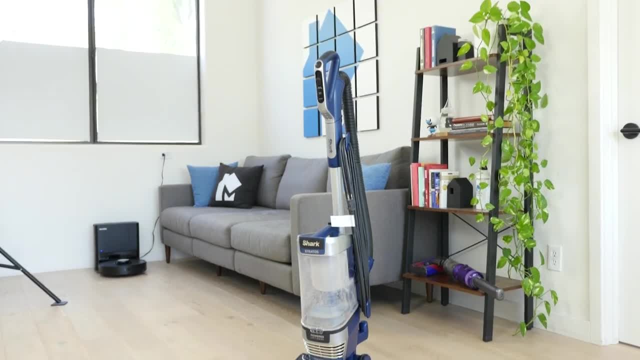 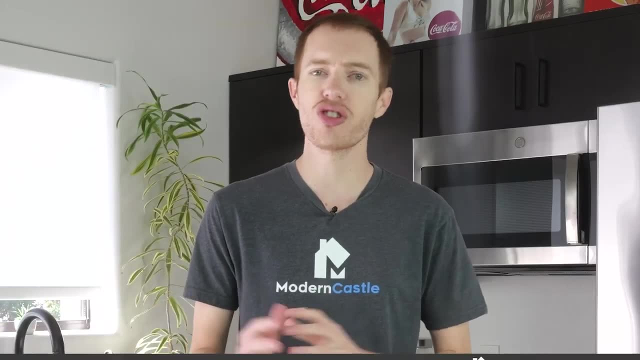 has few weaknesses and many strengths, making it a fantastic pick. While the Dyson Ball Animal 3 and Shark Stratos Upright are the current leading models from these manufacturers, there are a number of other slightly older models that are still fantastic: The Shark Apex, Shark Vertex. 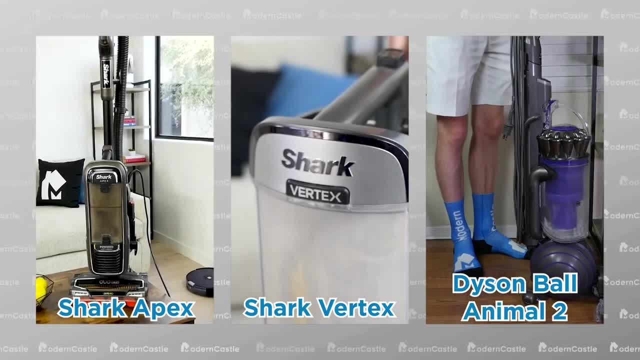 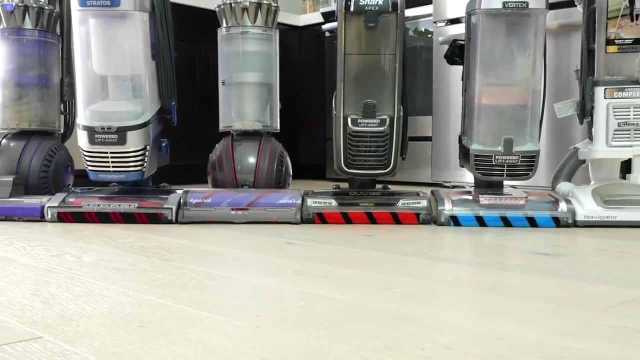 and Dyson Ball Animal 2 all have excellent cleaning performance, but may lack some of the newer features. That said, even with the newer upright vacuums, the prices can fluctuate. If you're looking for the most bang for your buck, we recommend checking out all of these models and seeing which. 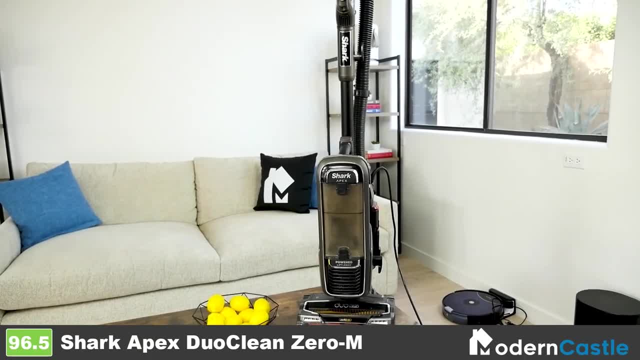 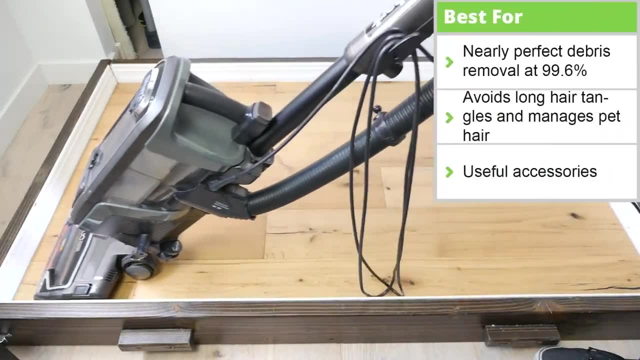 has the best price at that time. Despite being an older model than the Stratos, Shark Apex is still a fantastic upright. It removed 99.6% of all debris, had practically no long hair left after cleaning and minimal amounts of pet hair. It packs a completely sealed 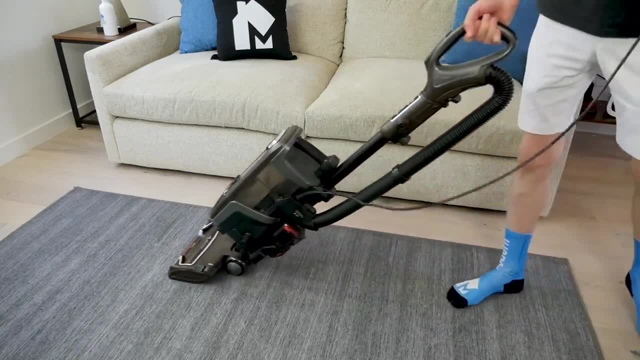 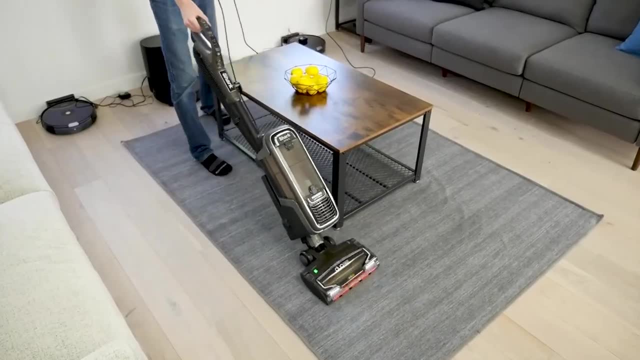 system with a 0.21 gallon dustbin and 30 foot cord. Additionally, the Apex has a washable filter and includes a pet hair tool to aid in pet hair removal. While it may lack some of the newest features we see on the Stratos, it's still a powerful contender and a great pick as an upright. 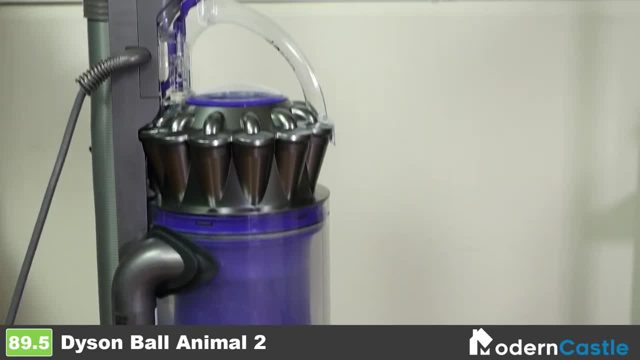 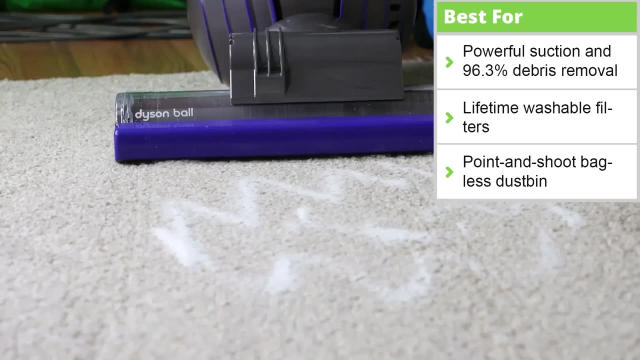 The Dyson Ball Animal 2 is still one of the most powerful upright vacuums we've tested to date. It had so much suction that it had minor issues getting on top of the cereal on high pile carpet. Despite that, it's a fantastic performer. 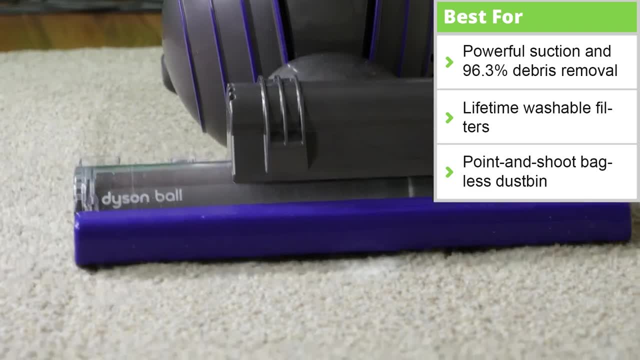 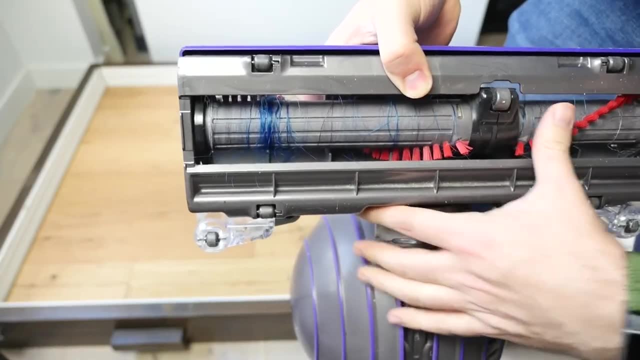 removing 96.3% of debris across all floor types. Pet hair wasn't an issue for the Animal 2, although long hair was more of a serious concern. 48% of the long hair tangled in our tests, but it was fairly easy to remove. In addition, the dustbin was mostly sealed, leaking some smoke. 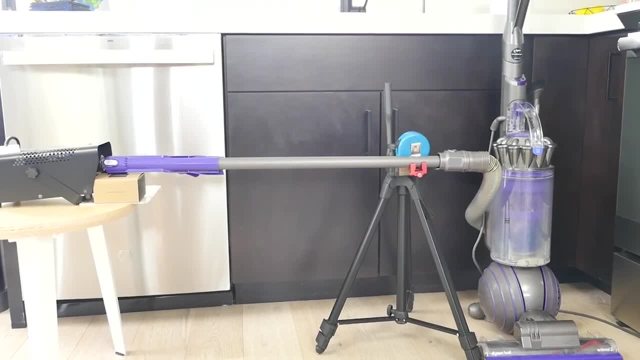 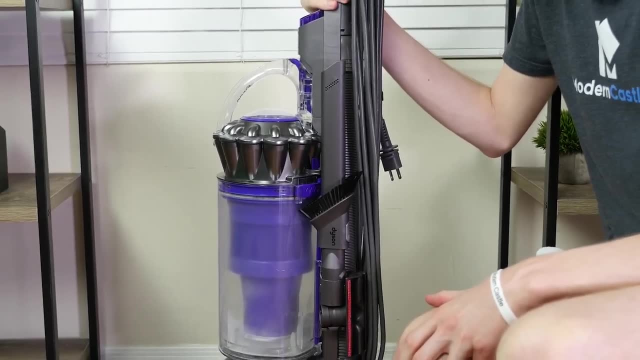 from our smoke machine. That said, we believe it's not enough to warrant significant concern. Most likely the seal has weakened over years of use in our lab, as the Animal 2 has been in service since 2018.. Despite these minor issues, the Animal 2 is still a high performance, upright vacuum and 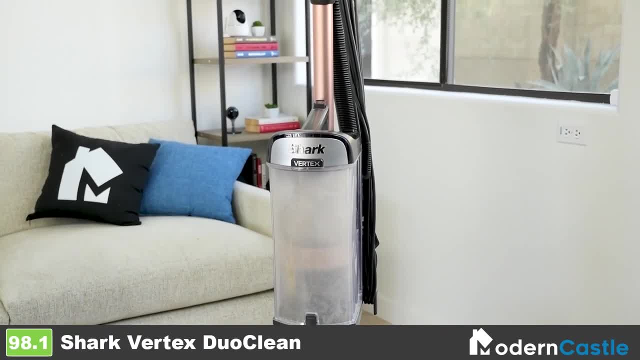 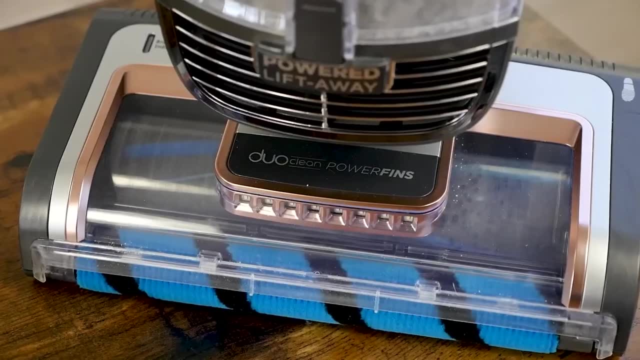 a good pick. Being an older model, you can see the evolution of the Shark Vertex Duo: clean to the Stratos. It has a lot of similar features we see in multiple Shark uprights, paired with excellent performance. Additionally, it introduced the improved power fins which replaced the more 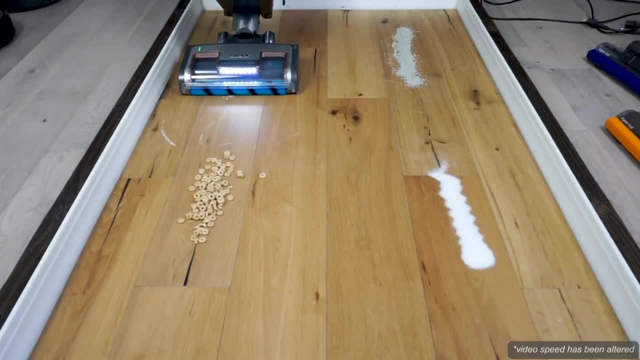 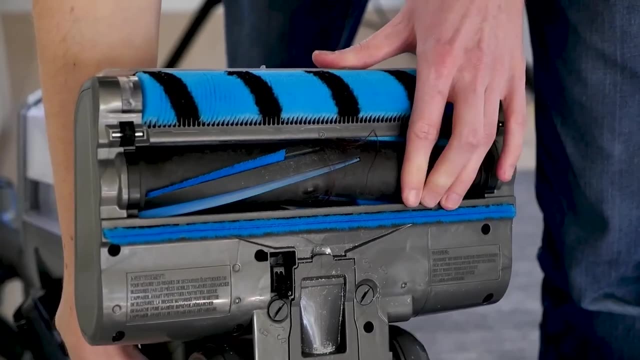 traditional bristles from the previous version. In our test, the Vertex showcased excellent performance across the board. It removed 99.4% of debris across all floor types, had no issues with long or pet hair, and removed the debris along edges and crevices. Furthermore, the device is 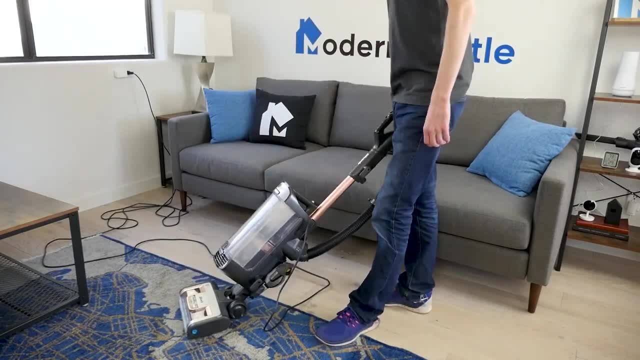 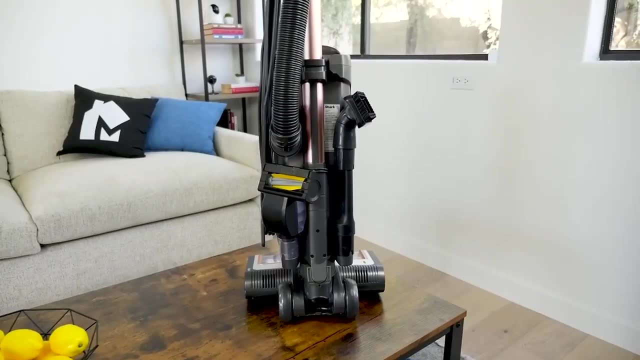 completely sealed. It packs a 0.24 gallon dustbin and 34 cord, giving it a healthy amount of reach while cleaning. It has the lift-away features, a soft roller brush on the front and comes with a number of useful accessories. All in all, it's a solid recommendation. if the 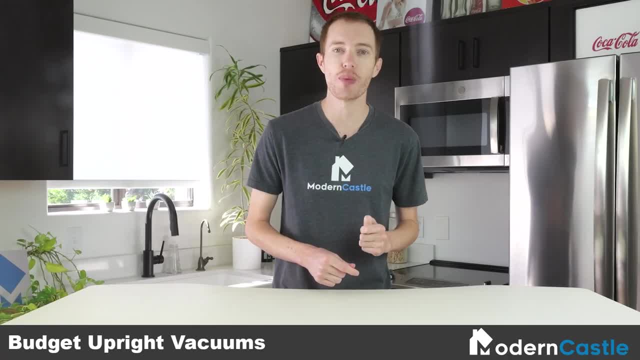 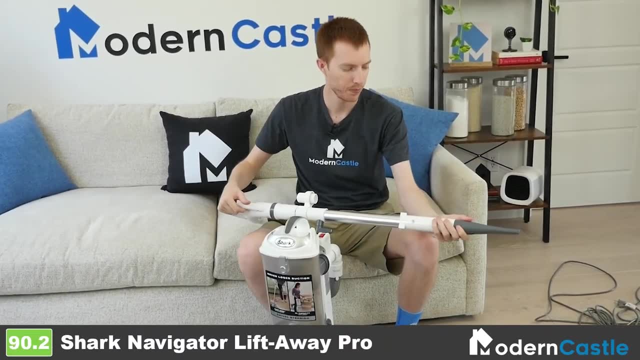 price is right. Finally, let's take a look at the least expensive upright vacuums on the list that still pack great performance. Due to its age and price, the Shark Navigator Lift-A-Way Pro has some shortcomings. It had lackluster performance on high pile carpet only removing 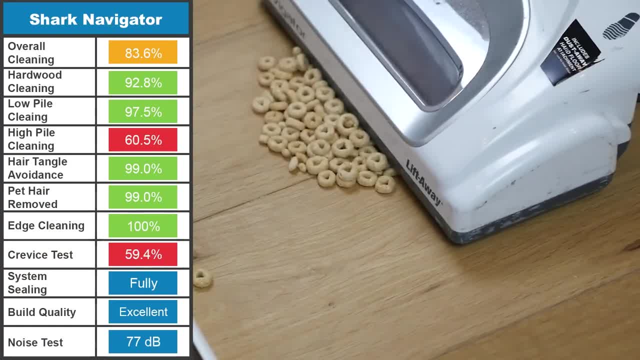 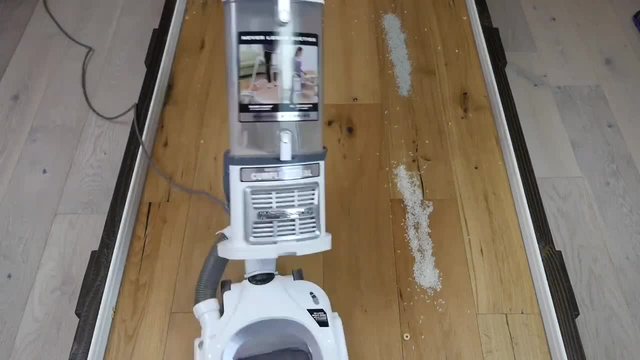 60.5% of debris. This is largely due to the height of the brush roll, which is a harder time of getting on top of cereal instead pushing more of it forward. Looking at other floor types, it showed great results On both hardwood and low pile carpet. it removed 92.0% of all debris. 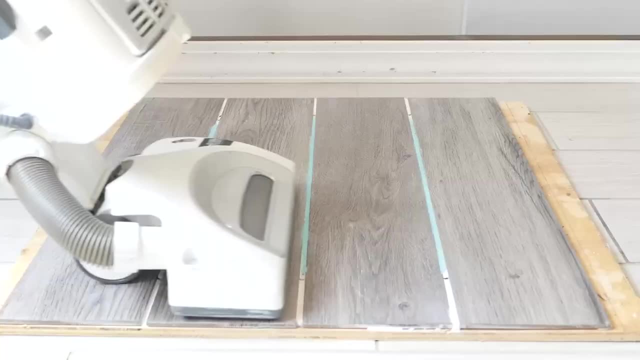 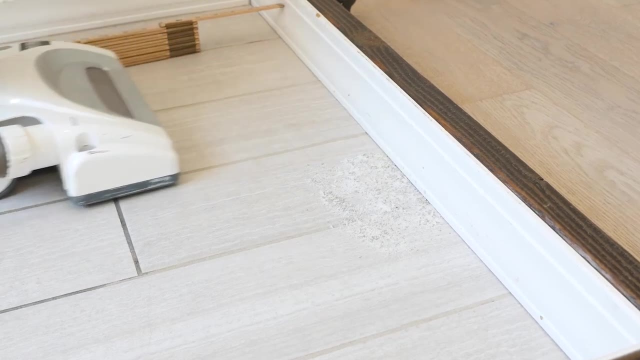 In addition, it managed long and pet hair with excellent results. While it had no issues with debris along edges, it did have some issues cleaning in crevices Across the board. in our crevice test only 59.4% of debris was removed, but that was with just a single forward and backward. 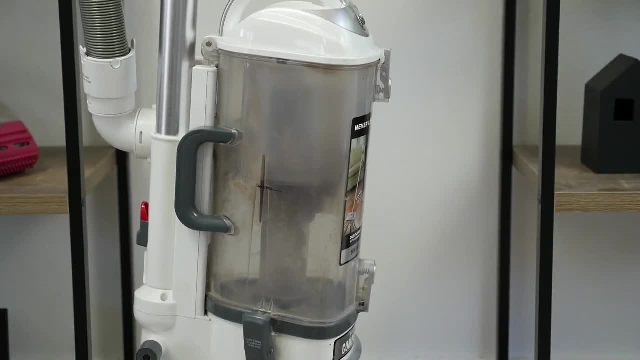 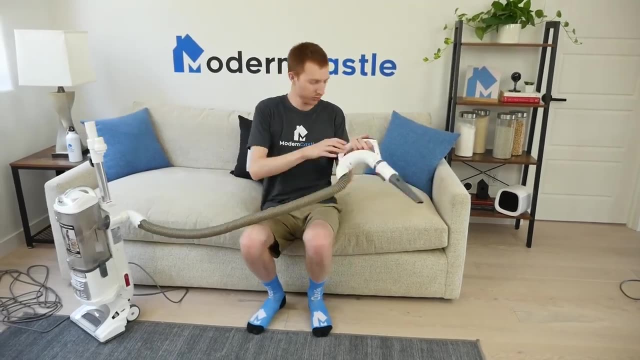 pass. Additionally, the Navigator has a 0.55 gallon dustbin that is completely sealed, paired with a 30-foot cord. It comes with some helpful attachments, like the pet power brush, and has the ability to lift away. like many other Shark uprights, It's not perfect. 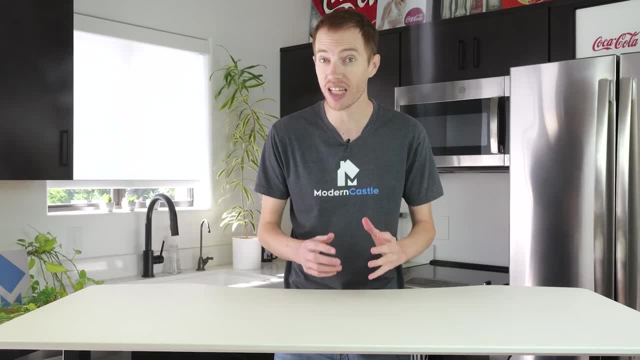 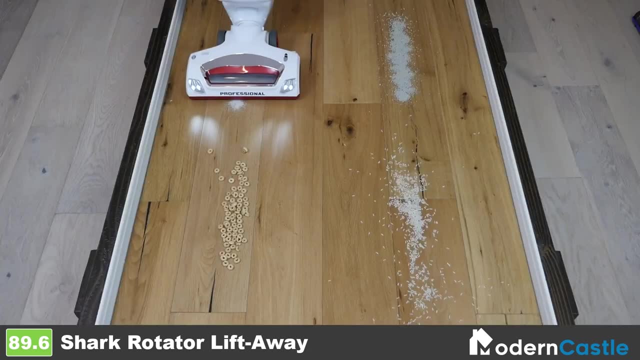 but considering how inexpensive it is compared to many other upright vacuums, it is an excellent deal in our view. Similar to the Shark Navigator, the Shark Rotator Lift-A-Way isn't perfect. While it removed 86.4% of all debris from all floor types, it did have some struggles with cereal. 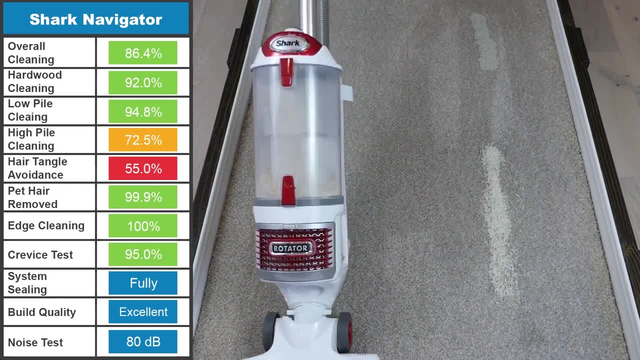 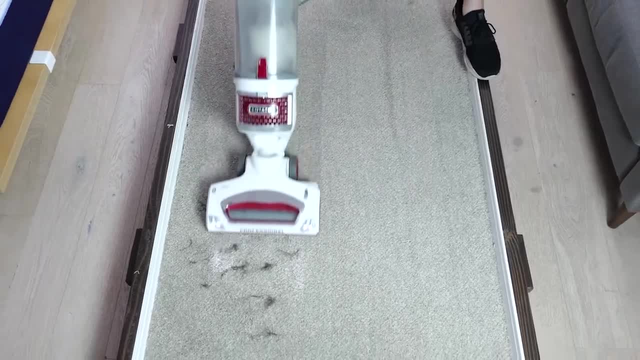 especially on high pile carpet, where it struggled to get on top of the debris. In addition, almost half of the long hair was tangled around the brush roll. However, pet hair posed no issue and practically all of it was removed. The good news doesn't stop there. 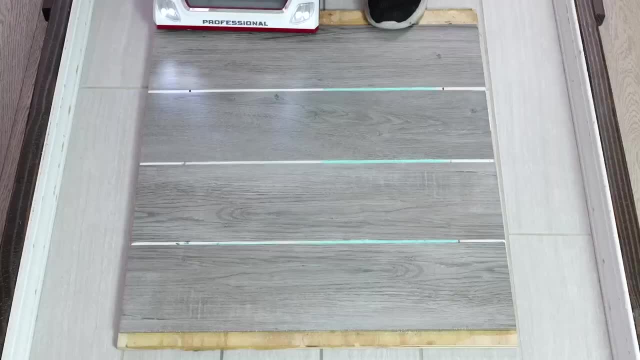 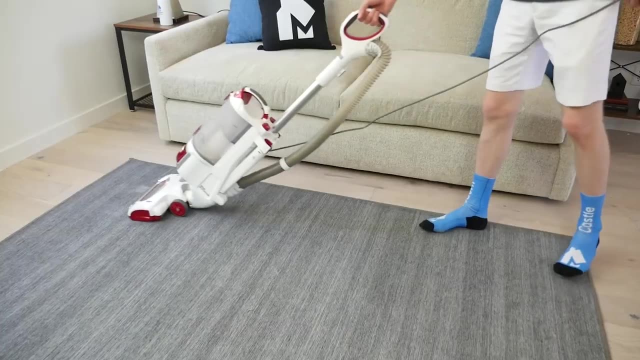 as the Shark Rotator was able to remove all of the debris from the edge tests and the vast majority of debris from the crevice tests. Additionally, the dustbin is completely sealed, ensuring no debris escapes while cleaning. It's equipped with a 0.33 gallon dustbin, has a 30-foot cord. 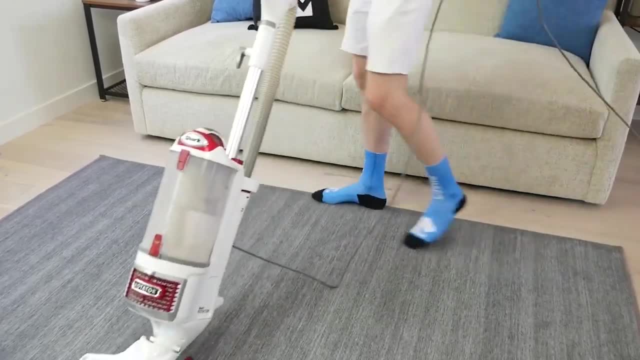 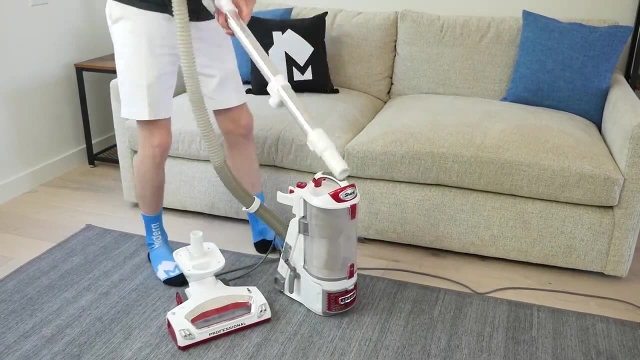 and is the second lightest vacuum on the list, with the lightest being the Shark Navigator. The Shark Rotator comes with a set of accessories, including the dust away tool and pet brush that all assist in different cleaning situations. Furthermore, the vacuum can double as a lift away canister vacuum when needed. 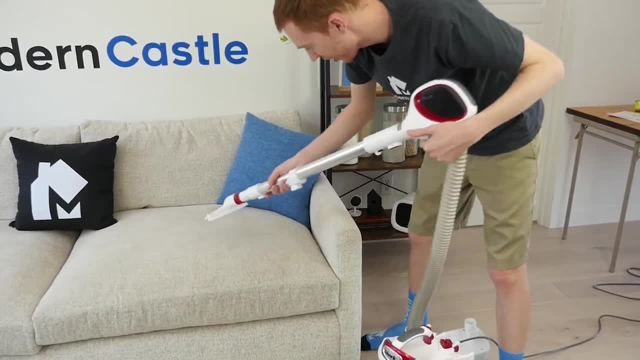 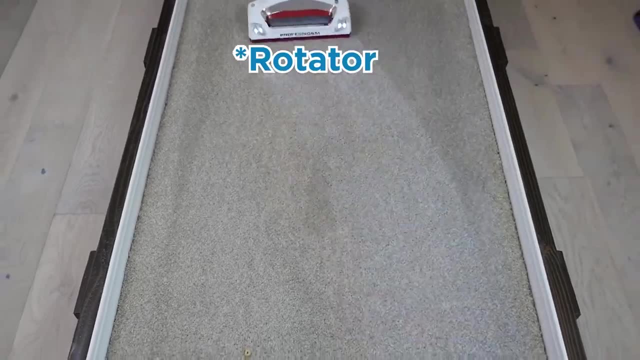 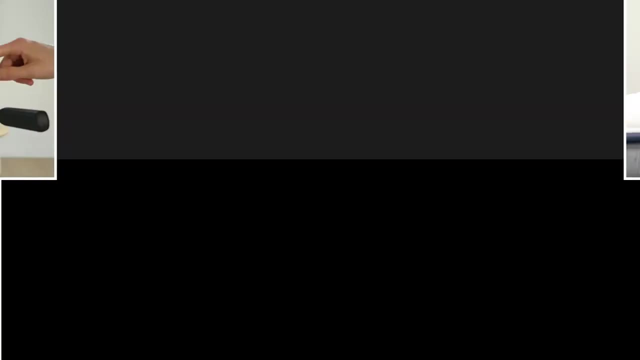 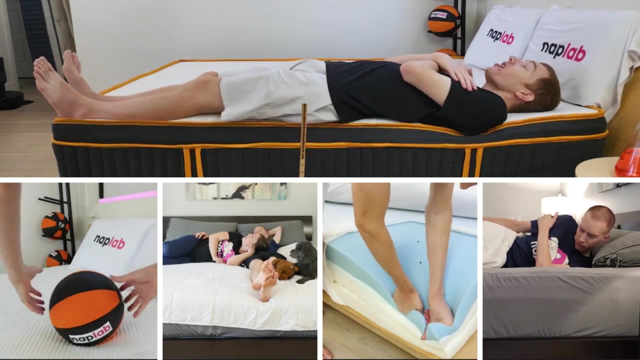 Again. the Shark Rotator lift away has its shortcomings, but despite these it still had relatively solid performance across the board. When we consider the price point, the Navigator remains an exceptionally good value If you're in the market for a new mattress and need help. 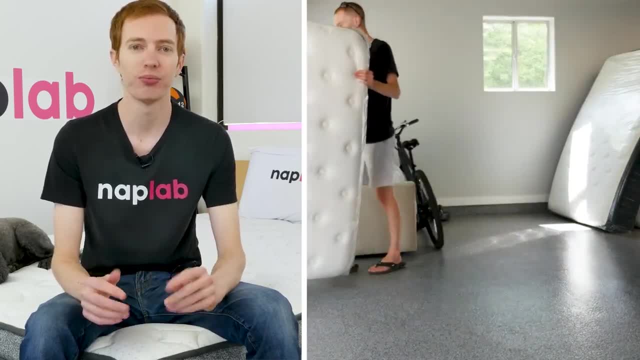 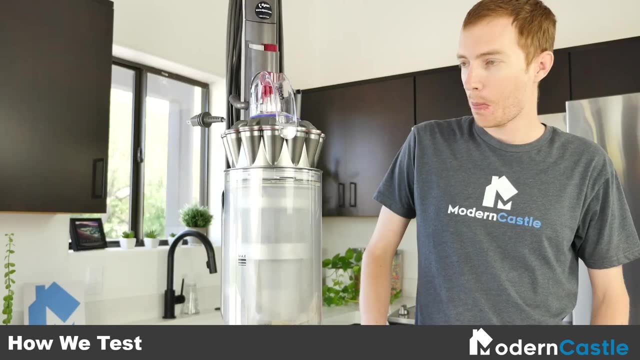 visit us over at KnappLabcom or on our channel at YouTube. We test and score upright vacuum cleaners using a battery of 11 data-driven tests. Our tests are a mix of objective data and subjective assessment, taking into consideration cleaner performance, build quality, system sealing, usability and maintenance. 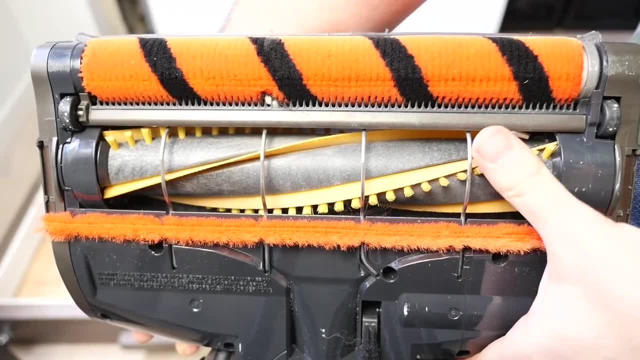 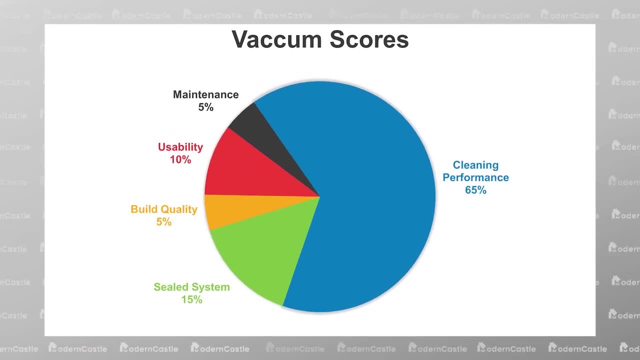 To choose the best upright vacuum. we base our selection on the top-performing and highest scoring upright vacuums according to our tests. These tests analyze the device's performance and are based on the test's performance and performance. Additionally, price and value were also taken into consideration. While there are other upright 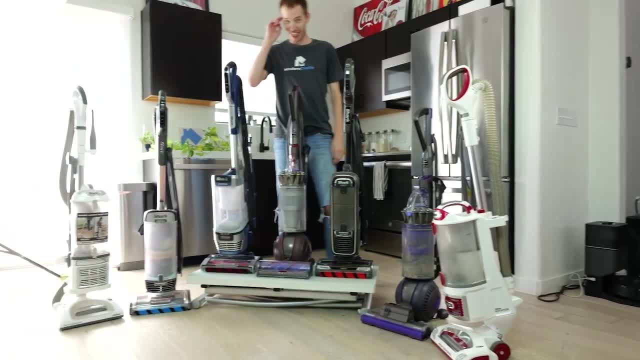 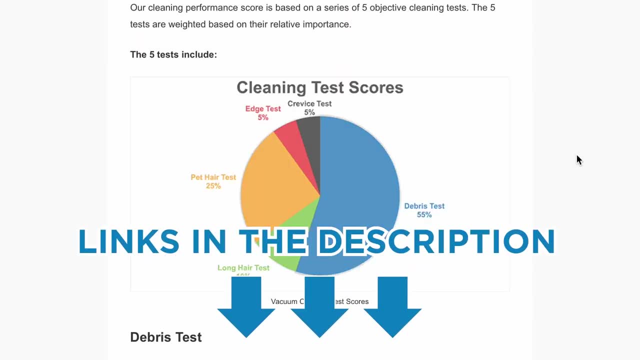 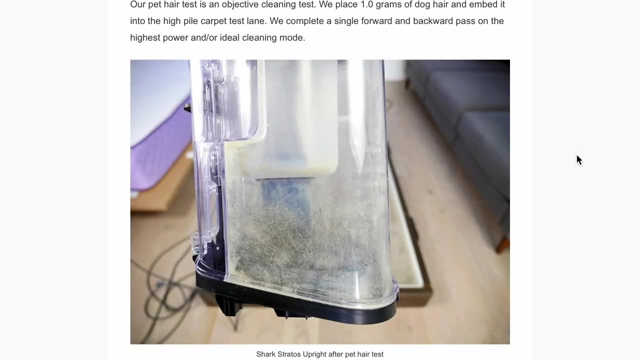 vacuums that could have appeared on the list. we wanted to include the best options available at a range of prices. Our testing process is detailed and rigorous. The links in the description have detailed write-ups and graphs to explain our testing process, scoring formulas and the criteria for how we choose the best vacuums. 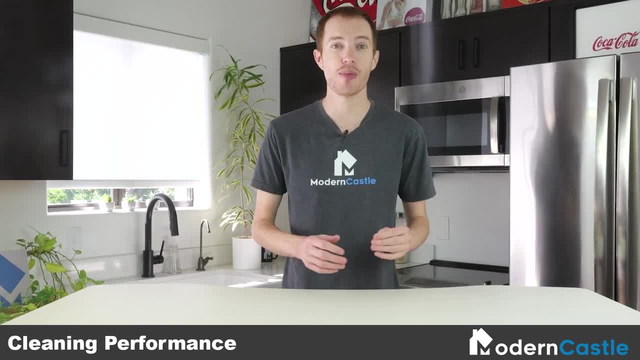 Cleaning performance for the majority of vacuums on this list is excellent, no matter the floor or debris type. The vacuum is a great option for cleaning your home or for cleaning your home. The vacuum is a great option for cleaning your home or for cleaning your home. This vacuum is a good 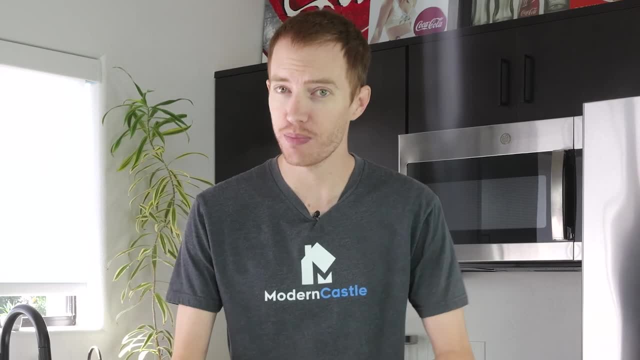 vacuum for cleaning your home. The vacuum is a great option for cleaning your home. The vacuum is a great vacuum for cleaning your home. The vacuum is a great vacuum for cleaning your home. However, there are some notable dips in performance, especially in regards to serial, the largest. 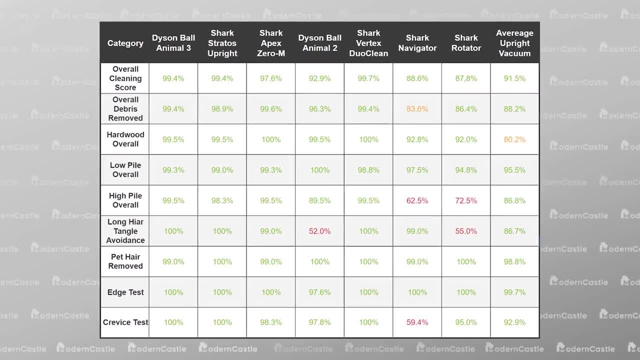 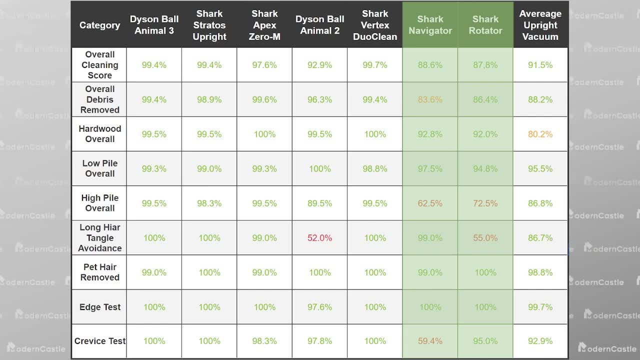 debris. As we can see from the data, the older and the cheaper the vacuum, the worse the performance generally is. Both the Shark Navigator and Shark Rotator struggle with serial on high-pile carpet, failing to get on top of the debris and instead pushing it forward. However, most newer models 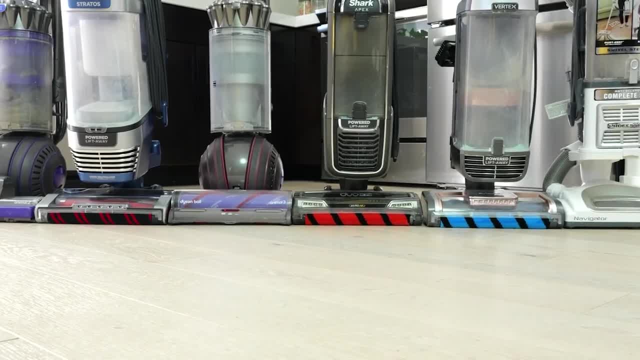 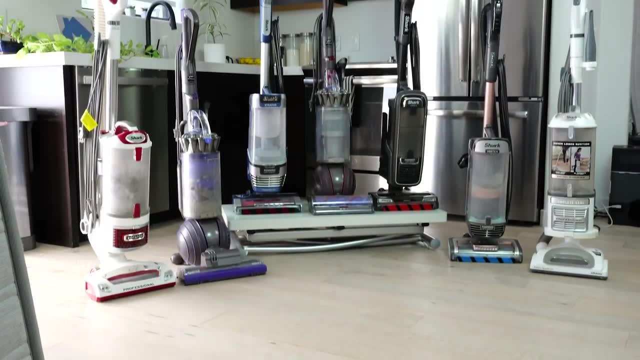 don't have this difficulty. On average, over the 23 plus uprights we've tested to date, vacuums are able to remove 88.2% of all debris. A few of the models are a little short of that mark, but the 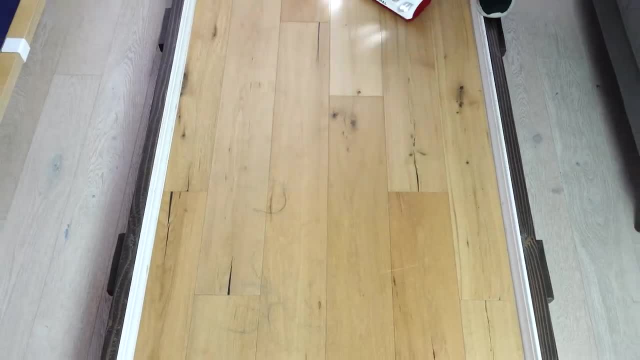 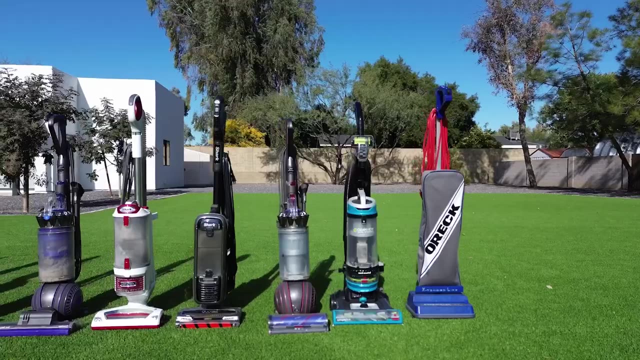 majority far surpass it. Long hair performance was also a struggle for the rotator, specifically failing to keep all the hair from tangling, Whereas the Navigator struggled with crevasses. However, all other vacuums on this list had nearly perfect performance across the board. 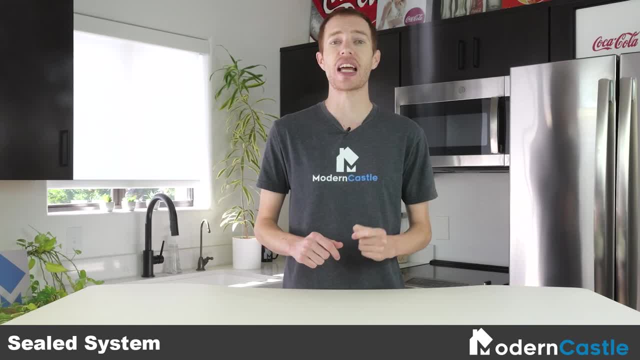 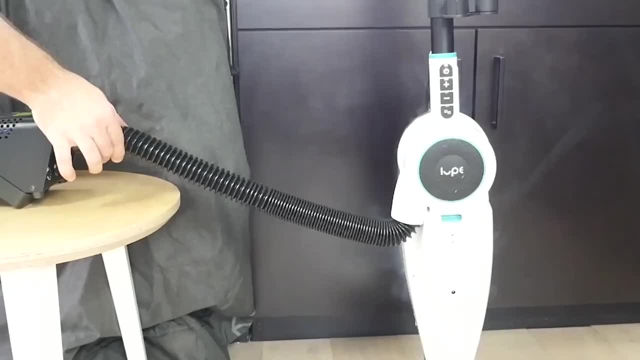 For the sealed system test. we want to determine how the entire vacuum system is sealed. Vacuums that are fully sealed ensure the dust and debris vacuum stay inside the vacuum. Vacuums that are not fully sealed may spread the debris around your home. 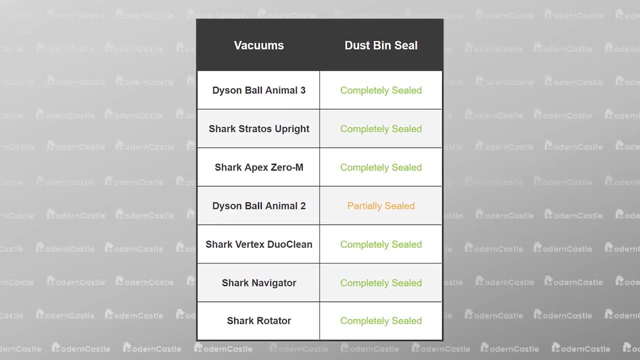 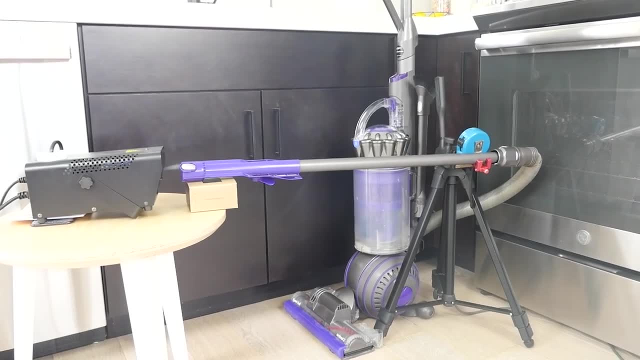 Most of the uprights on this list are completely sealed. That said, if you pick up the Dyson Ball Animal 2, we found it to just be partially sealed. However, the sealing is still effective enough to not warrant significant concern. In our view, the sealing on this model. 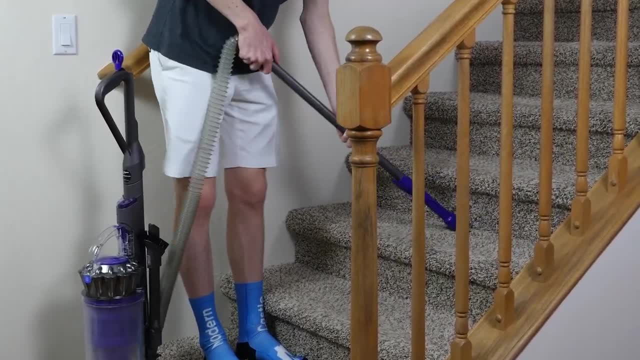 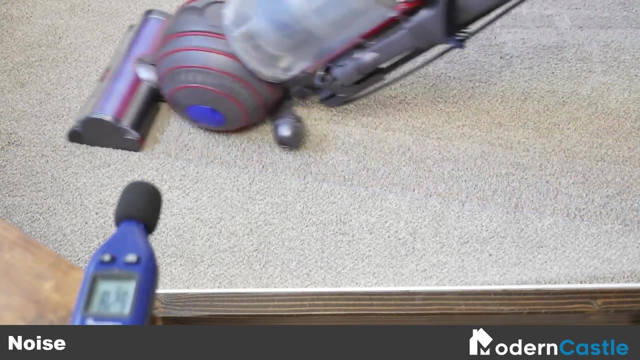 has likely weakened over time as it is among the oldest and most used vacuums in our studio. To measure how loud an upright is while in operation, we run the device in each power mode on high power carpet. Using a sound meter, we measure the level of noise. 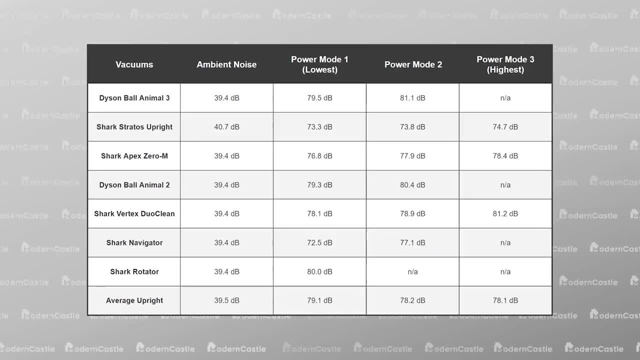 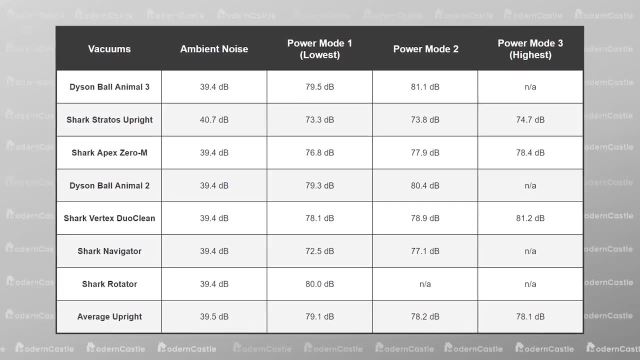 generated from about three feet away. There isn't much variance in the noise levels of the vacuums on this list. They all have noise levels in the 77 to 82 decibel range, with the Shark Navigator being the quietest at 77.1 decibels. 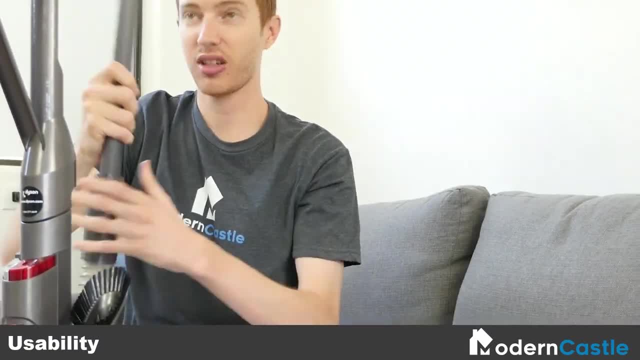 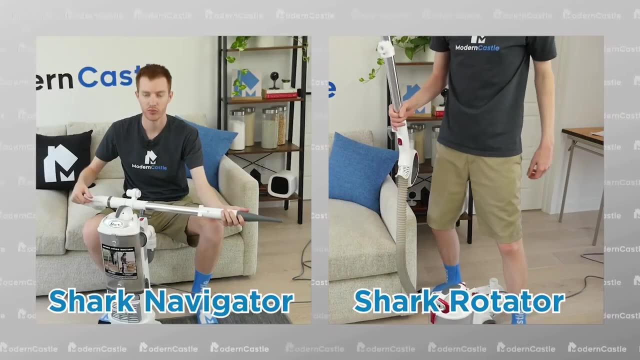 Usability is excellent for each of these vacuums. They each come with a range of attachments and accessories that aid in different cleaning situations, and they have pretty good maneuverability. That said, the Shark Rotator and Shark Navigator do feel a little stiffer than the other vacuums on this list. 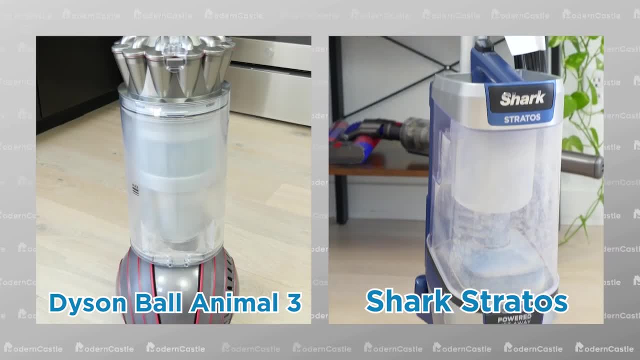 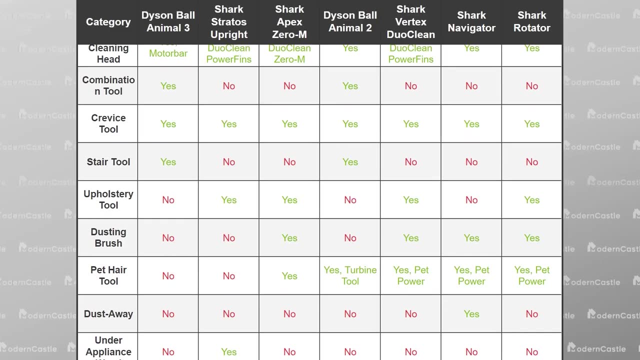 It's easier to make tighter turns with the other vacuums, like the Dyson Ball, Animal 3 and Shark Stratos. All in all, the difference is there, but it isn't massive. The table on screen shows which features and attachments. 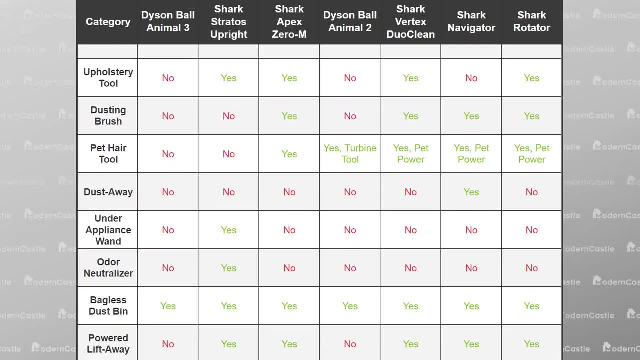 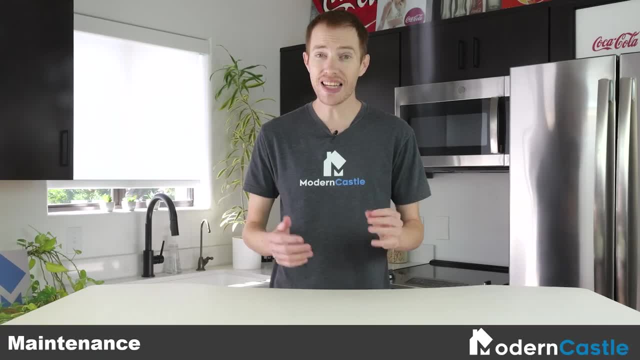 are included with each vacuum. Please do keep in mind, though, that some of the vacuums have multiple variants that may come with different set of accessories, attachments or in different colors. Maintenance is similar for all of these vacuums. 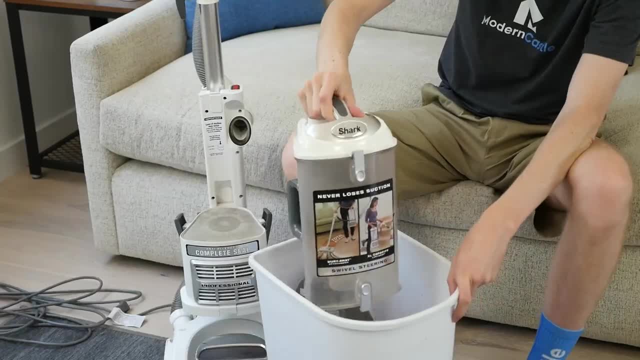 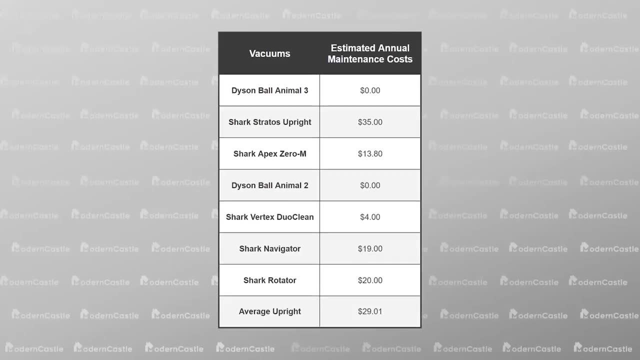 You will need to maintain the device, wash or replace the filters and keep the dustbin empty. The most notable difference is that the low-end models have filters that need to be replaced rather than washed. This increases annual maintenance costs, which are already relatively low for an upright vacuum. 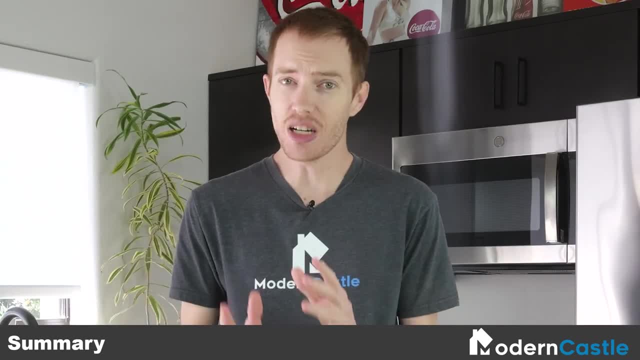 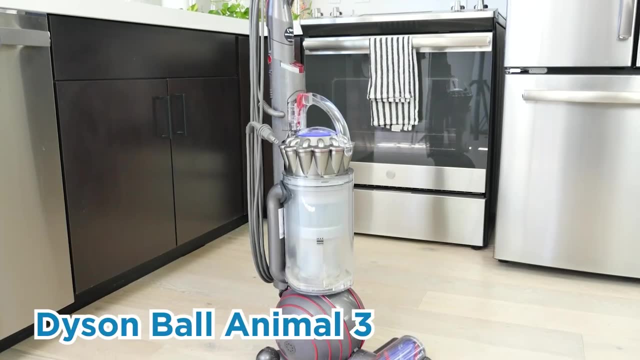 So which upright vacuum is best choice for you? While price is an important factor to consider, there are other key factors that set these vacuums apart. The Dyson Ball Animal 3 is a powerhouse of an upright vacuum. It can be the most expensive vacuum at times. 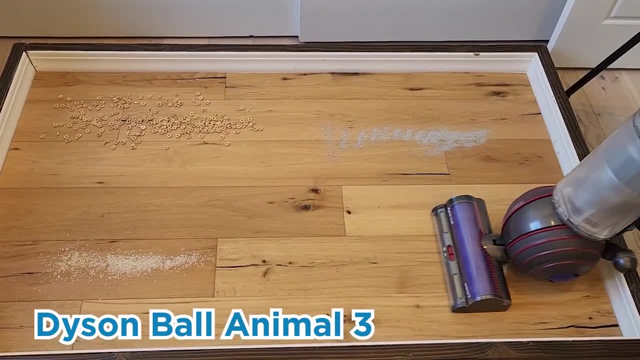 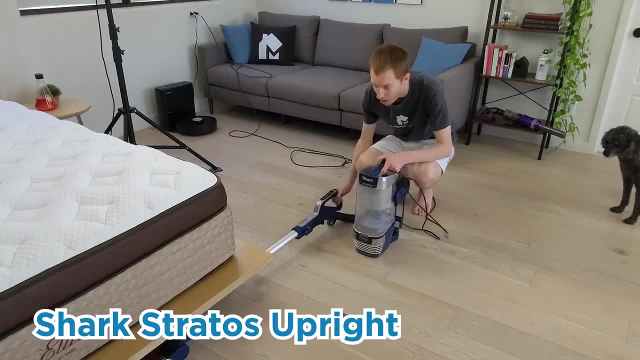 but its nearly perfect performance across the board make it an easy choice if you want the absolute best. The Shark Stratos upright is only slightly behind the Dyson Ball Animal 3, and in some situations, even better. It offers more maneuverability with its lift-away feature. 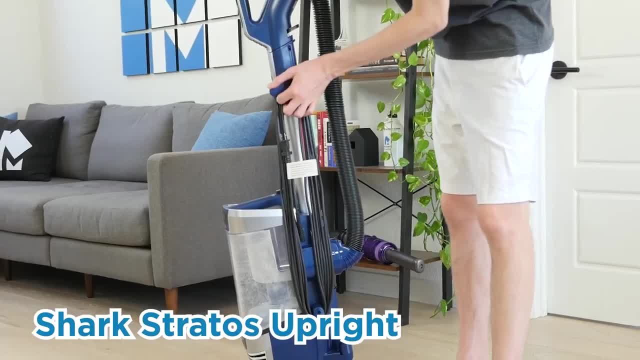 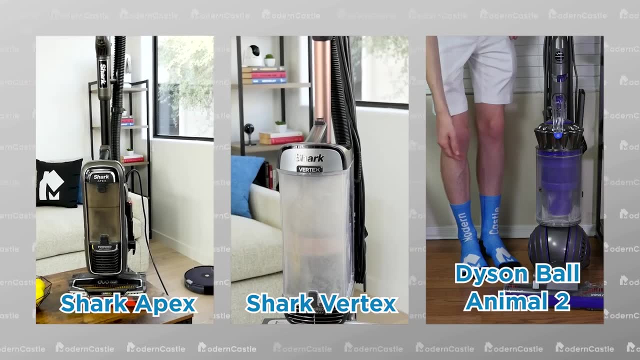 and masks unwanted odors with the odor-neutralizing pods. It's another incredibly powerful vacuum with improved usability. The Shark, Apex, Vertex and Dyson Ball Animal 3, are all great alternatives to the other high-end Shark and Dyson vacuums. 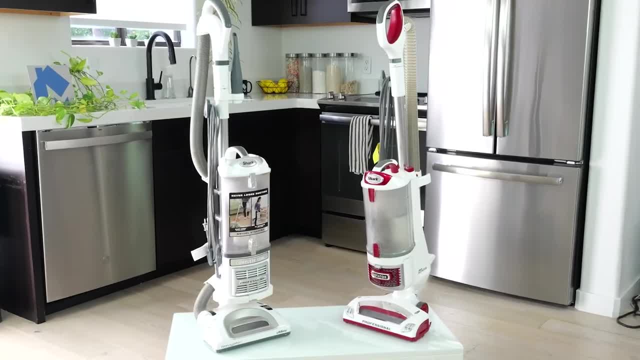 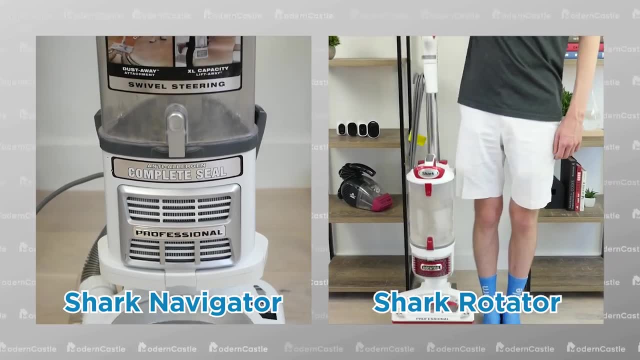 The prices can vary thanks to sales and general interest level, so if you want an alternative to the more expensive, newer upright models, pick whichever option is least expensive. Finally, both the Shark Navigator and Shark Rotator struggled more in some tests. However, they are incredibly budget-friendly. 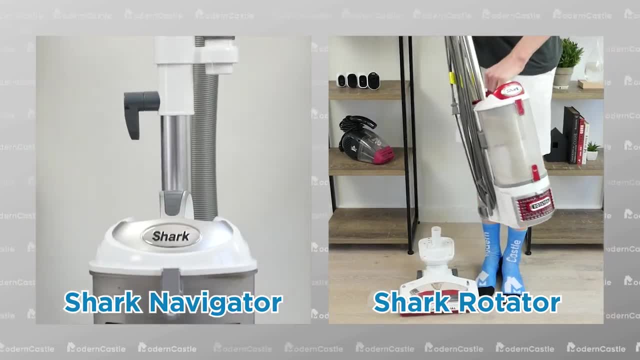 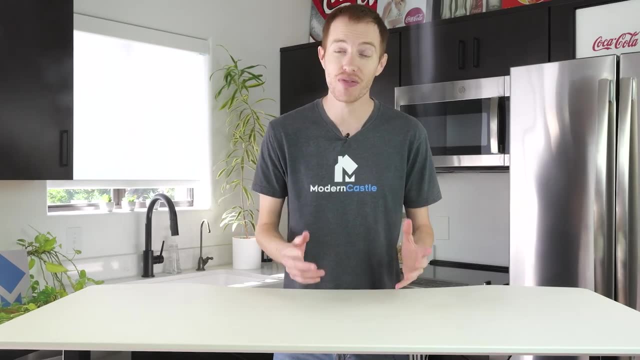 while still offering good enough cleaning performance for many homes. Well, guys, that's it for this video. I hope that it was helpful. Comments questions. please drop us those notes down below If you're interested in buying any of the vacuums.